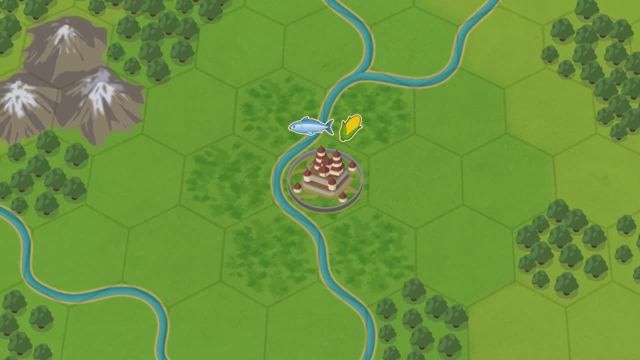 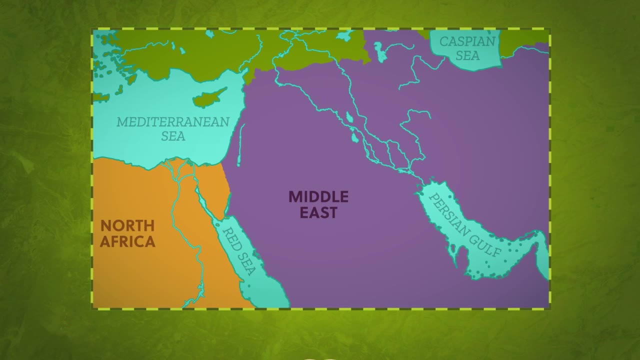 even food, like fish. but more important was the land alongside the river that holds water. when a river floods or overflows its channel, The floodplain Alongside rivers. agriculture bloomed in areas like the Fertile Crescent, in what we now. 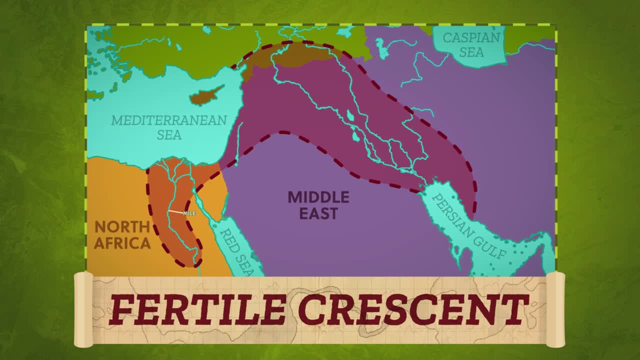 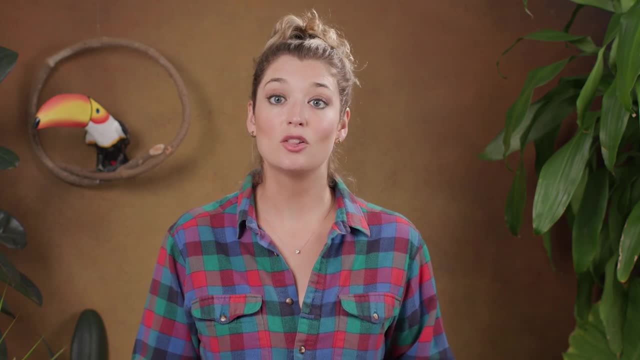 know as the Middle East and North Africa region. Regular floods along the Nile, Tigris and Euphrates rivers replenish the soil with nutrients, Which makes them perfect for growing some of the first wheat varieties, along with dozens of other foods cultivated for the first time. 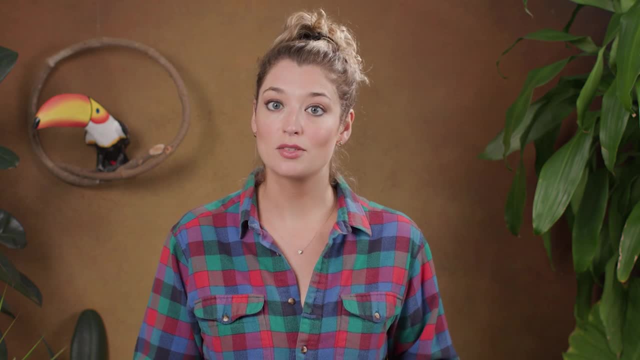 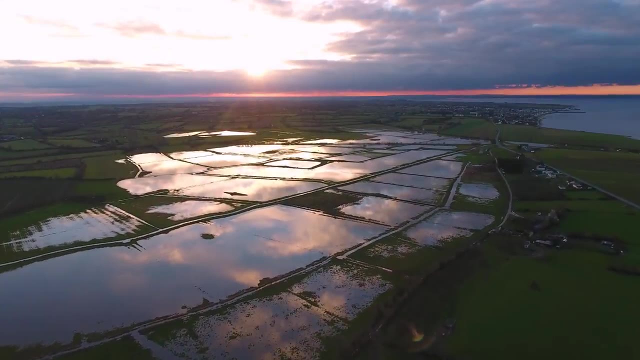 thousands of years ago, Floodplains led to a food surplus, which eventually meant not everyone had to produce food, which is really important for our communities today. But there's also a price for living on a floodplain: We have to contend with seasonal flooding or even catastrophic flooding. Of course, the most essential element of a river is well the water, And how much water is in a river is a key ingredient in flooding, which actually depends on where the stream gets its water. Stream levels can change as overland flow changes, which is water that flows over the Earth's surface from precipitation or snowmelt that doesn't infiltrate or absorb into the surrounding soil. But actually much of the base flow, or the average constant level of the stream, doesn't come over land. Underground water makes its way through soil until it reaches an aquifer. river, lake or ocean. So stream levels can change from the groundwater flow, which is the flow of water within the soil when the soil is fully saturated, And we have names for the different types of streams that receive mostly overland or groundwater flow. A seasonal or ephemeral stream will only have water if there's been 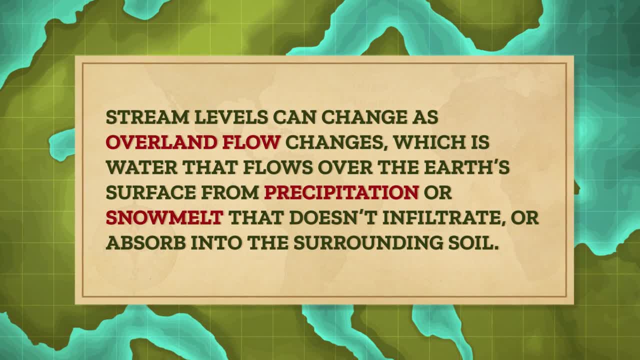 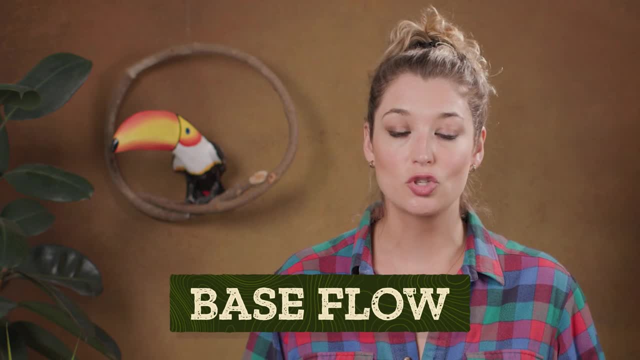 enough precipitation, But perennial streams usually flow all year and are fed by underground sources, Basically because of the way groundwater is stored and because it eventually gets evaporated. slower groundwater flow is more consistent than overland flow, which depends on the sometimes fickle precipitation. 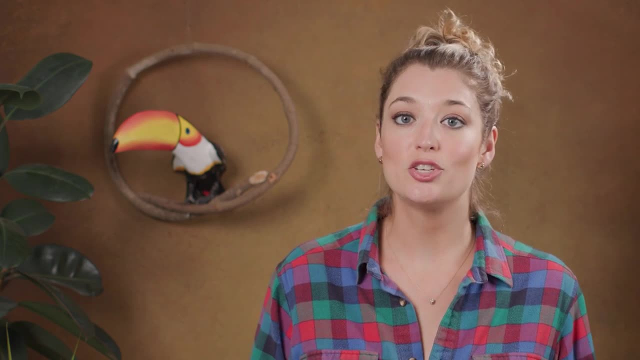 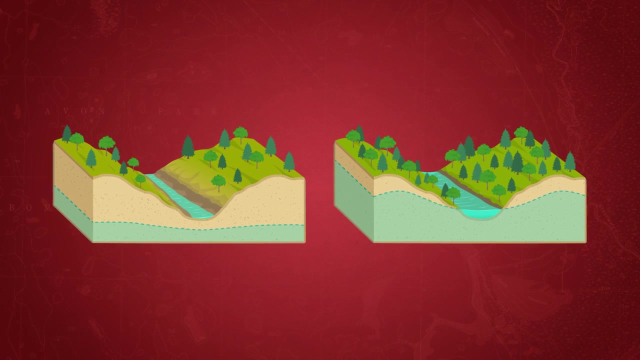 But if either of those sources suddenly increases, how much water is in the stream and how fast it's moving can also increase, leading to a flood. In fact, messing with these sources are fundamental ways humans can influence the flow of a stream, either accidentally. 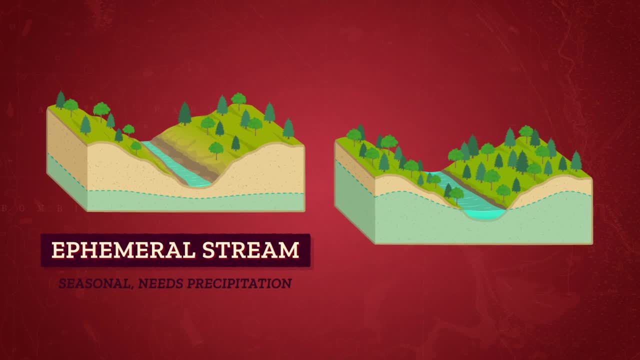 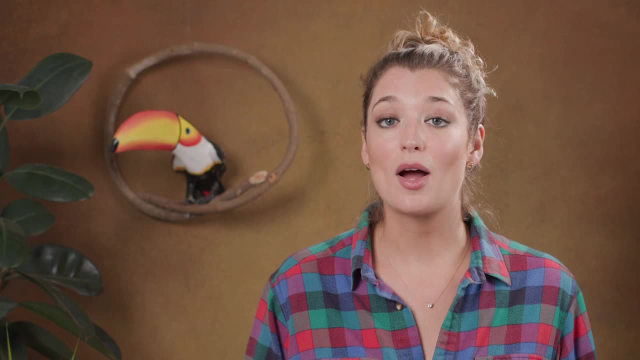 or intentionally So we have to be somewhat diligent To keep track of river levels, particularly after a storm. we can construct a hydrograph or a chart that shows how much water leaves a stream. With a hydrograph, we can understand how the stream responds to things like average. 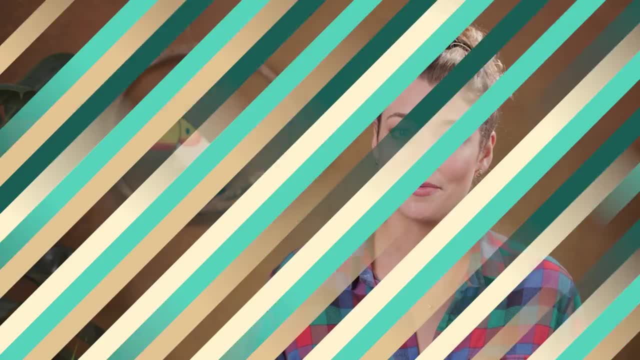 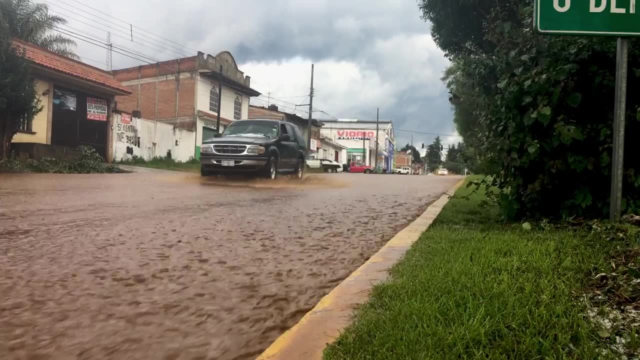 rainfall and snowmelt or tides and storm surges, And we can see how often those natural processes add a sudden influx of water to the stream and when that might cause a flood. Take, for instance, Indonesia, specifically the island of Java. Most of the rivers on 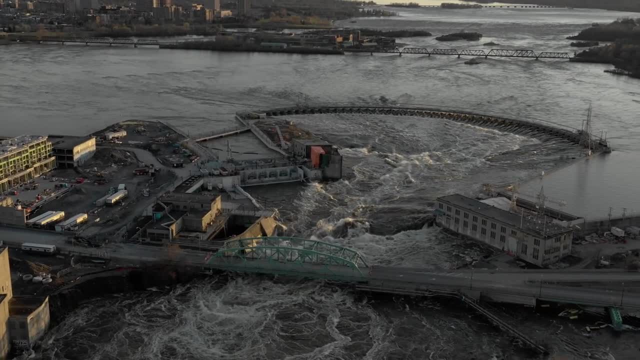 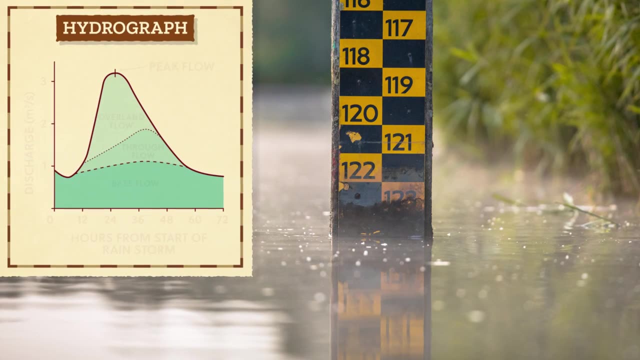 Java are seasonal because the island has distinct dry and wet seasons and a tropical monsoon climate. We can see from this climograph, which shows the relationship between two climate elements, that the wettest months are January and February, but rain is common from November to April. It rains more in the mountains, where the headwaters are, so even if there isn't a lot of rain at sea level, the people there can still be impacted. The river then has to handle all that water, Just like the geology of the basin helps decide.